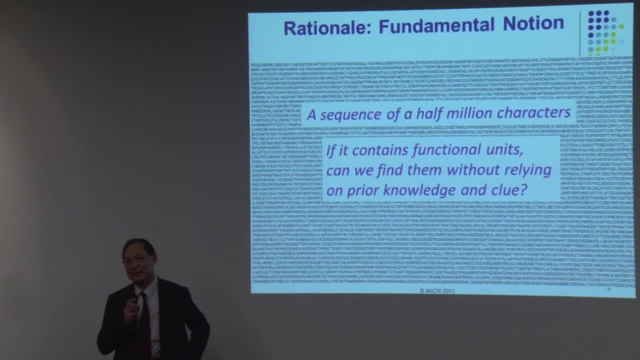 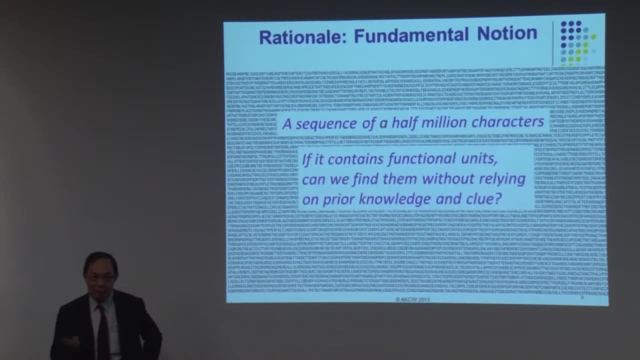 If there's some information embedded in some data, can we find it? Without prior knowledge, without any clue, can you find it? What does it mean? What does it mean from an entropy sense? If they are random, they are independent, they are equally probable. definitely nothing can be found. 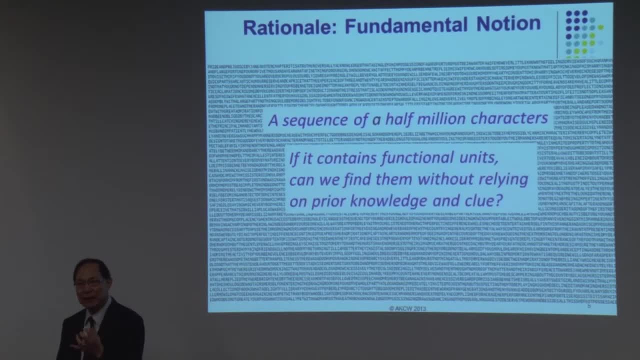 But if they contain meaning, if they are organized, if I can find out how they deviate from the default random, independent model, then at least I know that it contains something. You cannot consider it to be a reason from a random situation, And from that we begin to search a way. 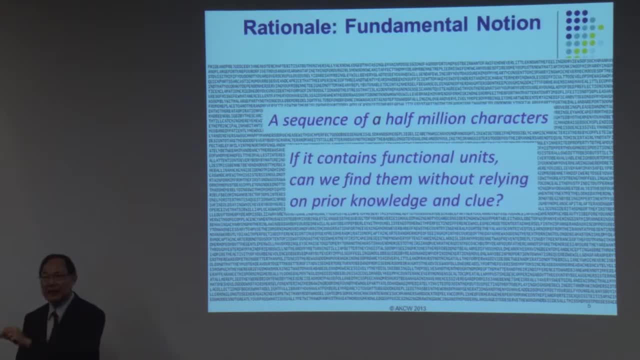 First, what is information? Can we know information here and there, And then we go one step further to find out not only a measure, but what exactly? Now take for example: suppose you are given a sequence, a very long sequence. 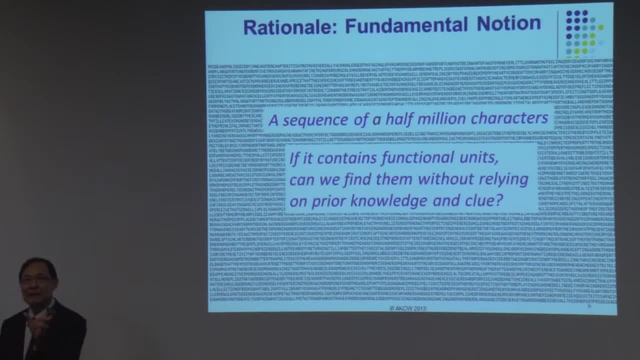 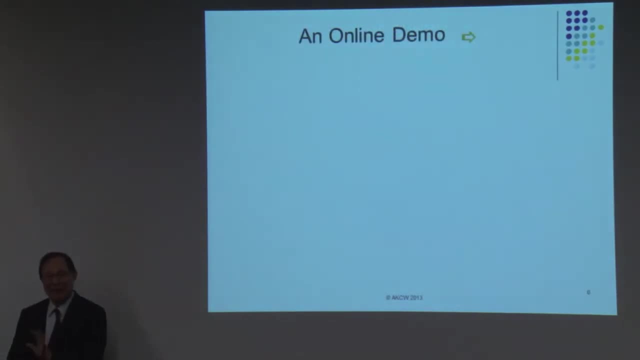 How many characters? If it contains some sort of sequence that has meaning, can you find it? This is very simple. Now, actually, I can give you a demo, but actually, because of time, within less than two seconds we can find out some non-random association of local sequence. 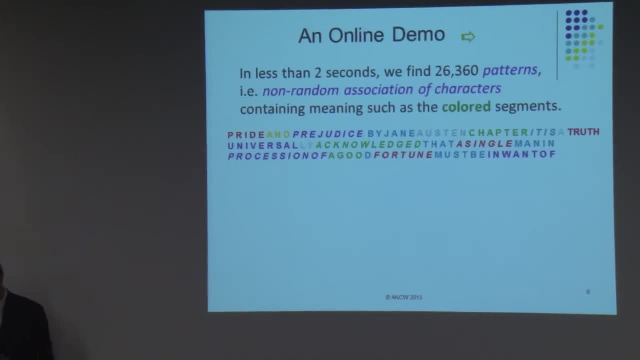 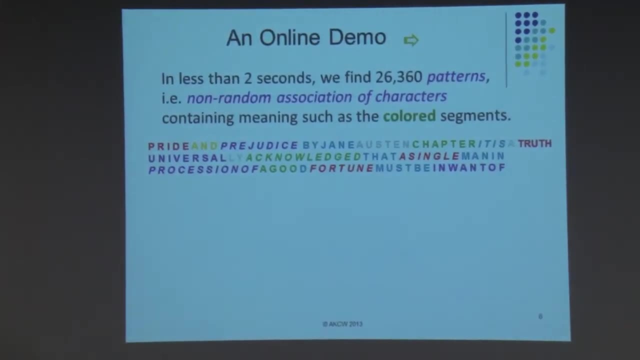 And what are they In this case? like pride, fortune and knowledge in one of. If I ask you, do they contain meaning? Unless you do not know English, you know they contain meaning. Why it is there? Why we can find it? 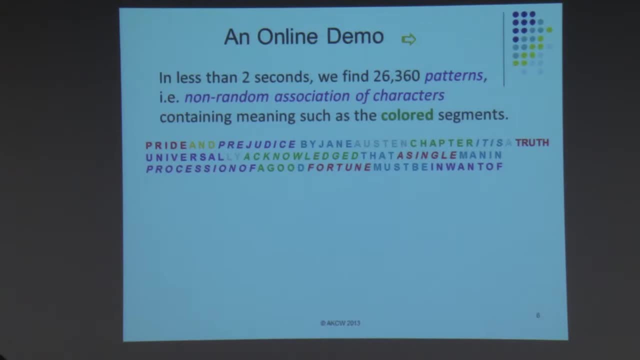 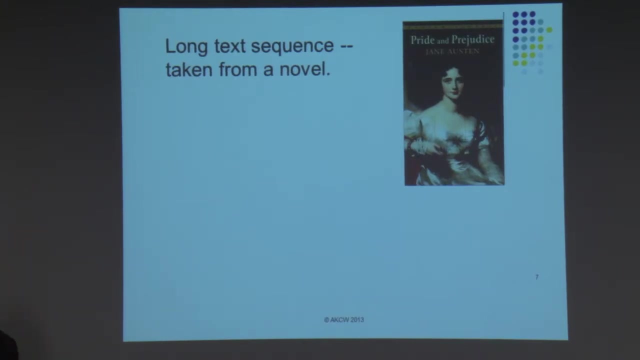 Because there is an English, there is a phonetic, there is a language structure behind language. So what are they Actually? when I first discovered binding site, my student asked me: how do you know that it is important? How about, let us give you some English example? 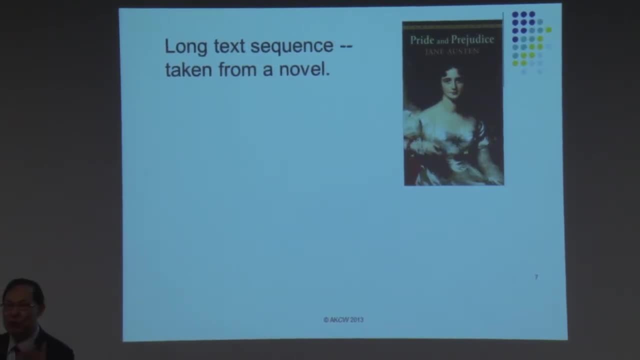 So we take the whole text of pride and prejudice. We remove all the punctuation, all the spacing, No uppercase and lowercase. So it is actually it is a half-million long set of sequence Again, in within two seconds. we found out that all the non-random 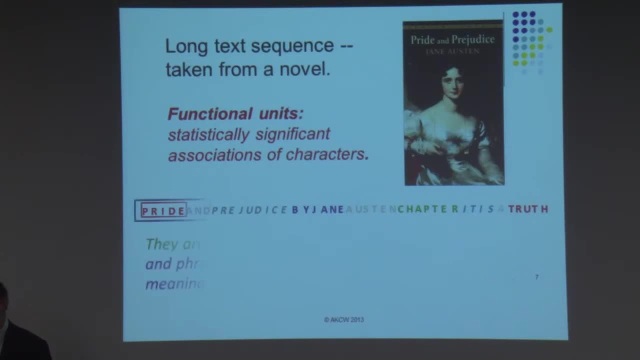 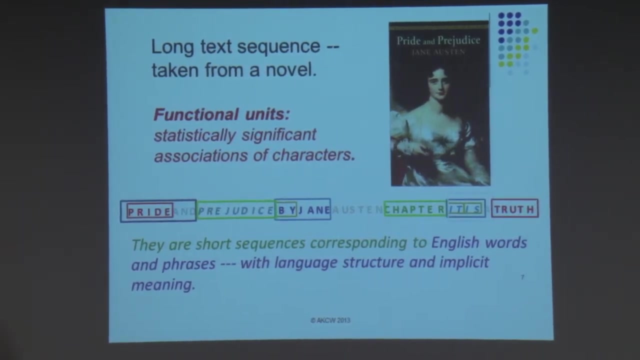 not independent kind of unit And it contains the data, the language structure, phonetic and everything all embed. They are short sentences, correspond to English words and phrases with language structure and implicit meaning. So when we apply the same technology to DNA. 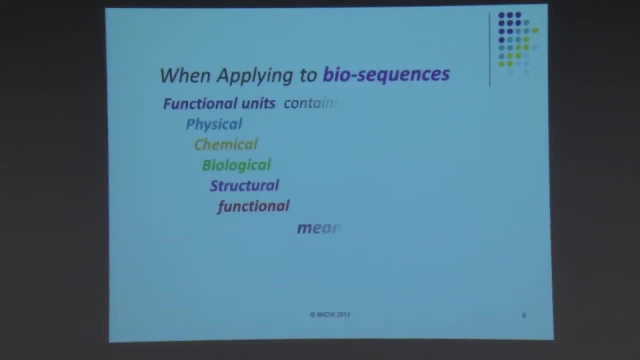 then we can find out the functional unit, which contains some kind of physical meaning, chemical meaning, biological meaning, structural meaning, functional meaning. Why? Because they are encoded for that purpose. So, when we apply this to the upstream of the transcripts, factor of DNA. 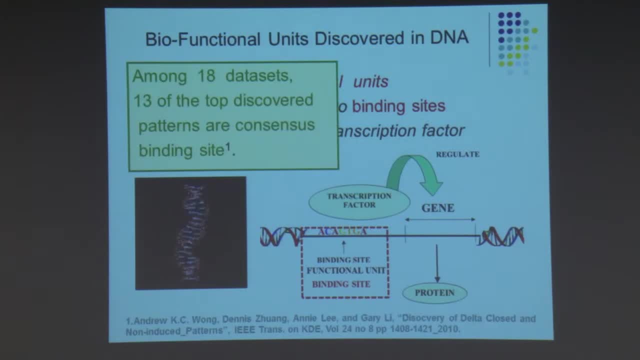 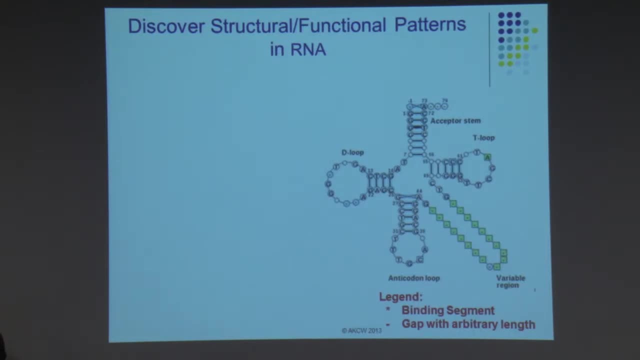 then, out of the 18 data sets, we found 13 of them. They are actually the binding site very high up. We also apply this to transfer RNA. We all know to transfer RNA is a well structure, Again without any prior knowledge or clue. 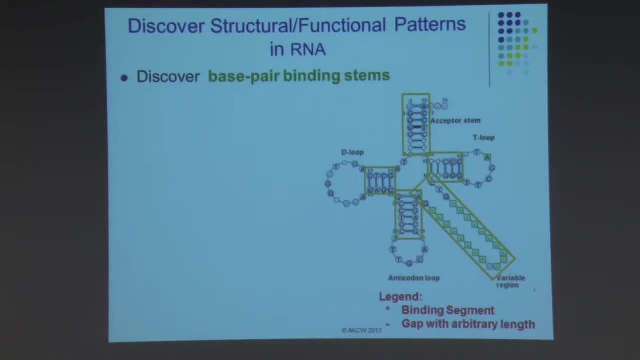 we are able to find out all the pair stem And beyond. we can also find out what we call a distant pattern. It means that they co-occur together in a molecule. Why they co-occur? Because they have. they are responsible for tertiary structure. 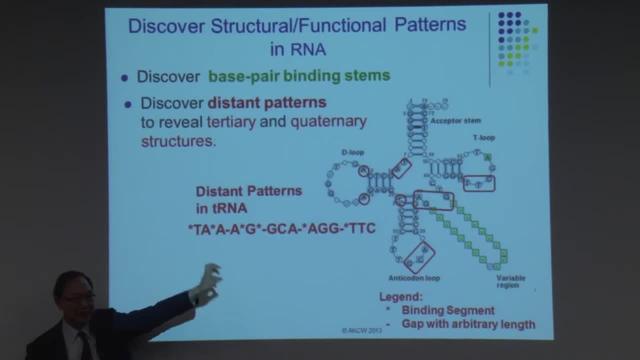 folding and many other things. It's embedded there, It's encoded there. So of course, we do not apply to transfer RNA. We have learned a lot about transfer RNA, But we can also apply to other ribosomes of RNA. 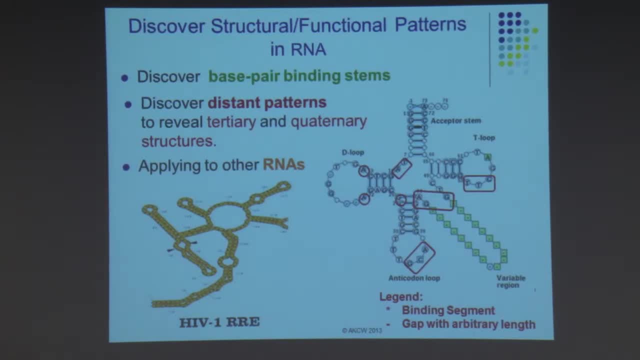 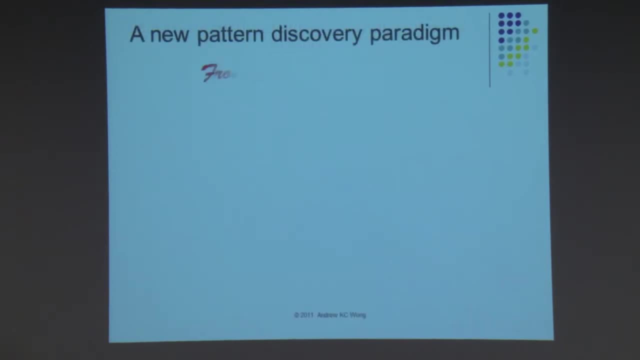 The whole idea is: no matter which is protein or RNA, DNA or language. as long as there is a functional meaning there, we will find it okay. So therefore, we propose a new paradigm. How can we move data into knowledge? 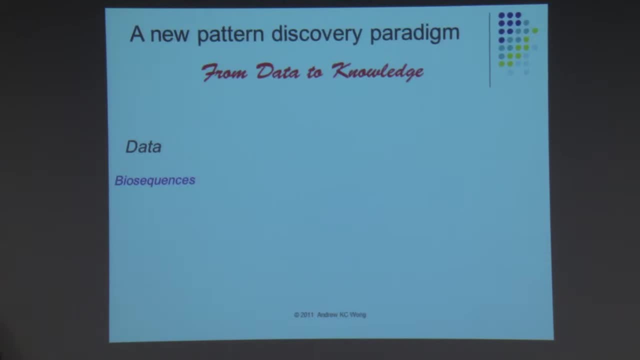 By data. definitely in a bioinformatics setting it could be biosequences, can be, microarrays, can be tables By pattern. we mean some association. They are not inter-association or relation or rule And if we represent it in a certain form, 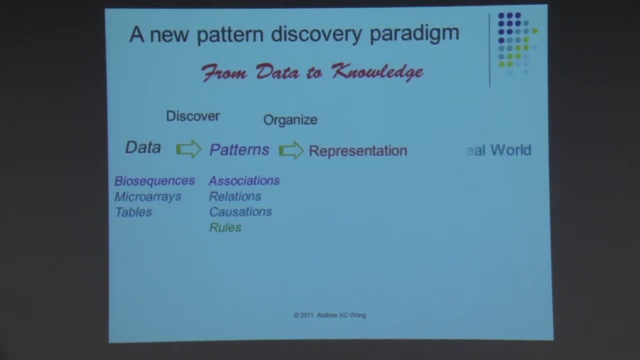 so that it can be verified from the real world through experimentation, through scientific application. explanation so that we can infer the structure and function. and perhaps, if we do not know those before and we find it and explain it, then it becomes scientific discovery. 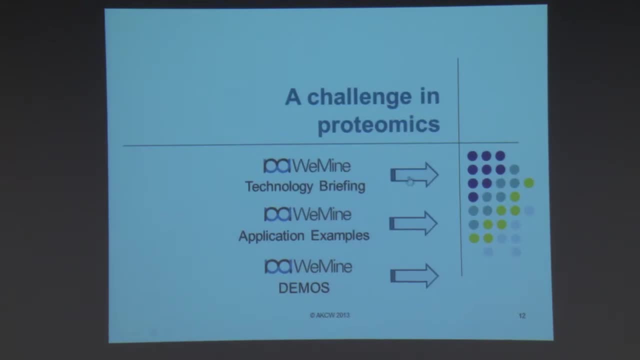 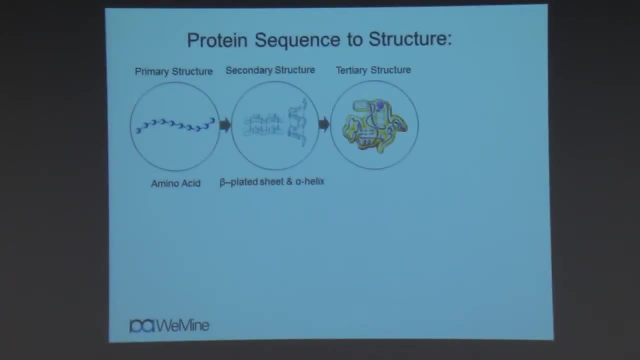 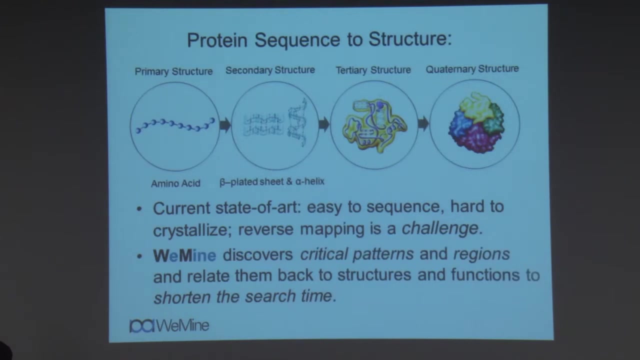 Now I want to give you a briefing of the technology behind. Now, first, protein sequence. We all know from a binary structure to secondary, to tertiary and then to quadrary. But the currency of arc is easy to sequence, particularly with the new next-generation sequencing machine. 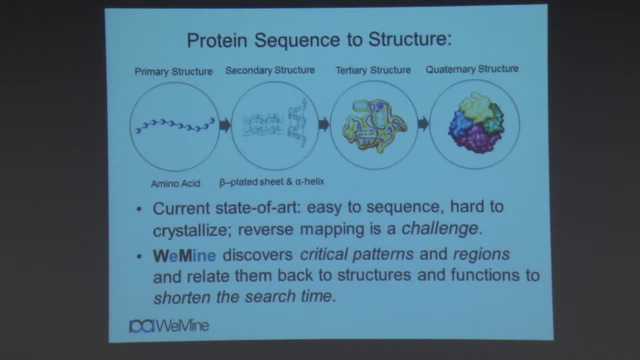 But hard to crystallize And reverse. mapping is very difficult From a 3D and going back to, let's say, at the primary structure and tell you right, it's not so simple. So we might try to discover the critical patterns and region. 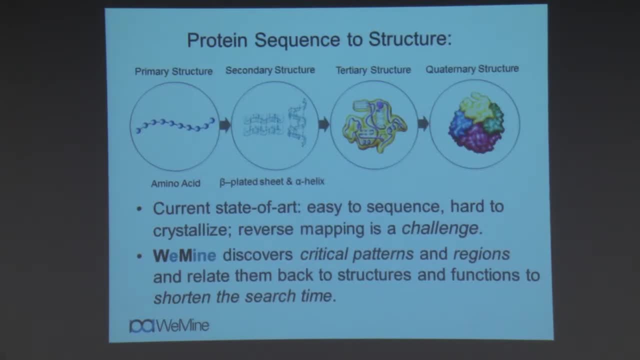 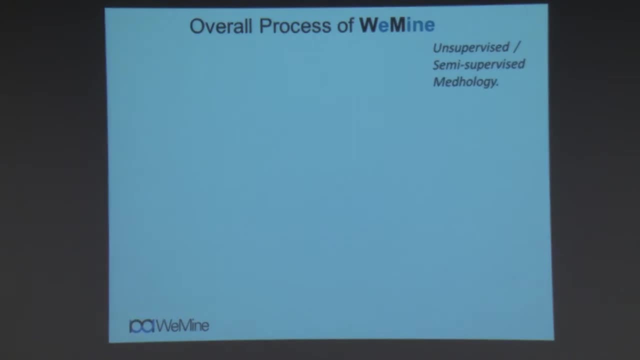 and relate them back to the structure and function. to shorten the search process, We have biologists, not replaced biologists. Now we can using ANSUBA. ANSUBA means that you do not need a pionautic. SUBA means that if you have a pionautic, you can use a pionautic. 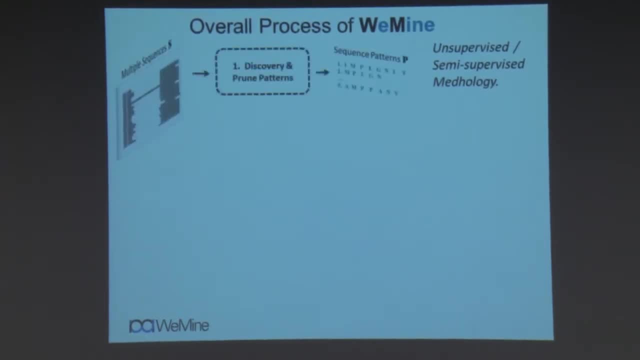 We begin with some kind of multiple sequences And then we discover and pull in the pattern By pattern. it means that they are sequence of association, not only pairwise, the whole, the whole word. okay, Then we align them and consider them. 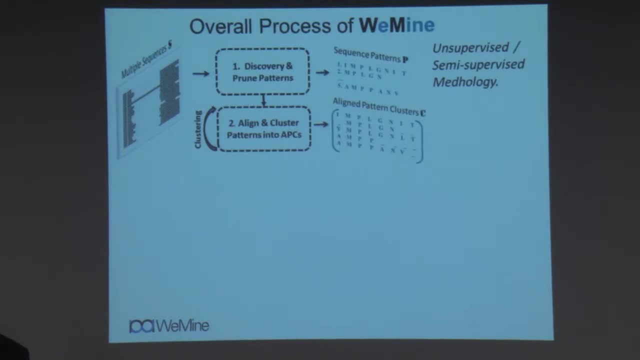 We bring the similar pattern together to reflect the local functionality And then of course we can go more further into the structure And then we can further partition the so-called aligned pattern cluster into sub-cluster When we bring something functional together. there are two issues. 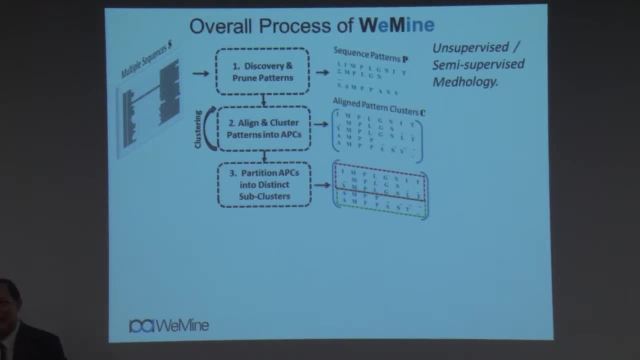 One issue: what are the functionality that govern that region And other? where are the discriminative information you can get to reflect the protein classes, protein group within the region? We localize it so that we are not talking about a whole molecule. We zero in to find out the functional region. 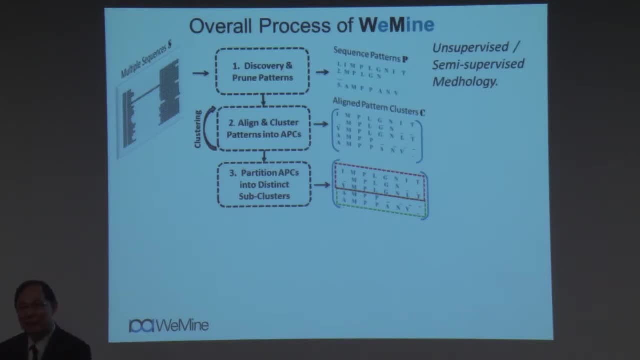 like a word, okay, Or a similar word, And then we can use the information to show: are they related back to the class characteristic of the protein? If we know that it is, we can explain, we can find some, And then we want to find out what pattern in those regions. 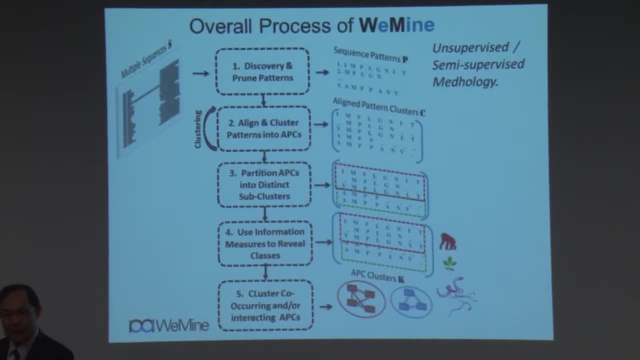 could occur on a sequence And what pattern in certain regions are interacting with other regions. There's a chemical kind of? if there is, then we can find out the interacting site. We can find out the site with the chemical and then we become a drug discovery. 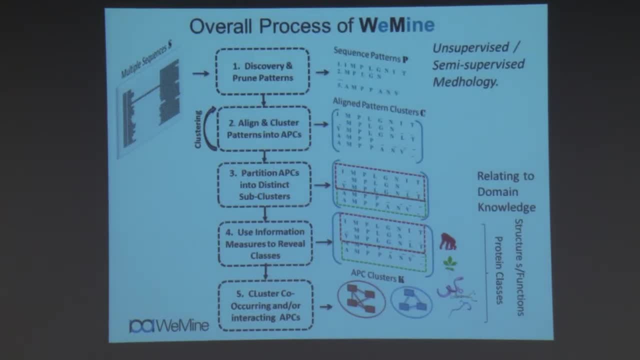 So the whole idea is: once we find out zero in this short sequence, then we can relate this back to the real world- the structure and function and protein classes, And then we can enhance it, but from the we bypass the bottleneck. 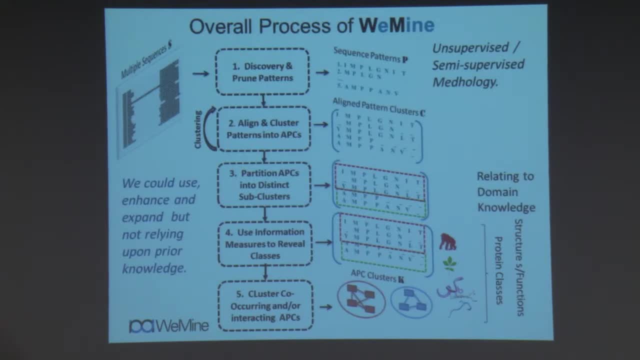 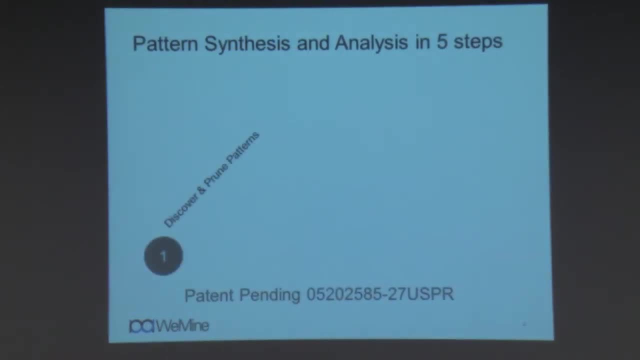 We don't need any prior law. Sometimes it's the prior law, it's the prior requirement that costs us time, Try and error, okay. So now we have five steps in this. First, we discover a prune pattern. Second, we align a cluster pattern into. 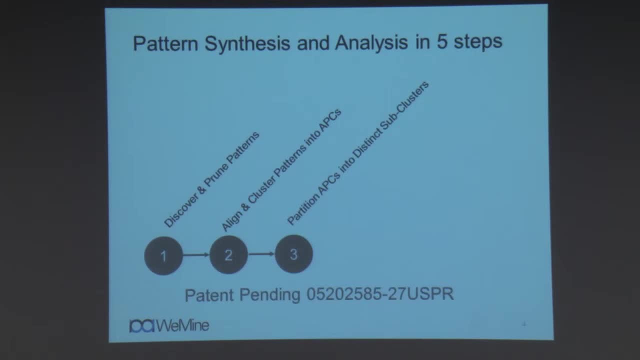 align pattern cluster And then we partition them into distinct sub-cluster to reflect their discriminability. And then we use information measure to review the classes so that we have objective places to show what are important, in what way. And then we discover co-occurrence. 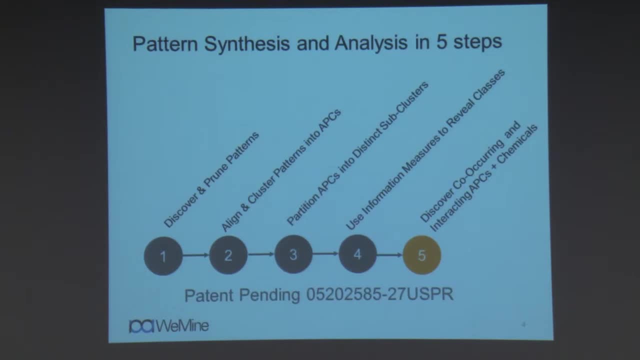 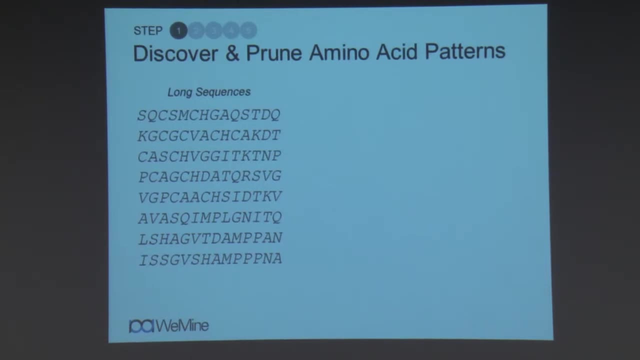 and also the interacting APC plus chemicals. Then now give an example. Suppose we have a long sequence of characters. we don't know what they are right, But by pattern we discover some association wherever they are. We don't need a consensus region, right? 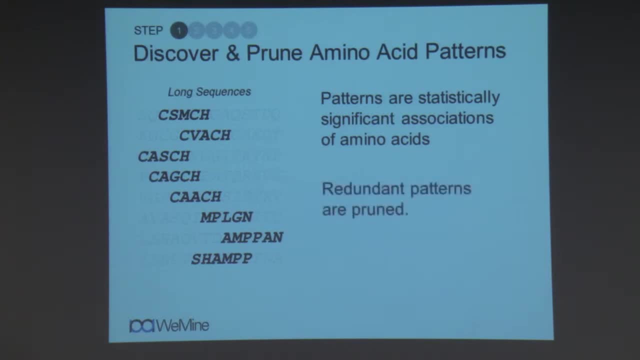 As long as they are similar, we can discover them, Then we remove the redundant pattern. If the super pattern contains a sub-pattern, its redundant is much worse. Now, then we align them. By alignment it means that we bring them into. 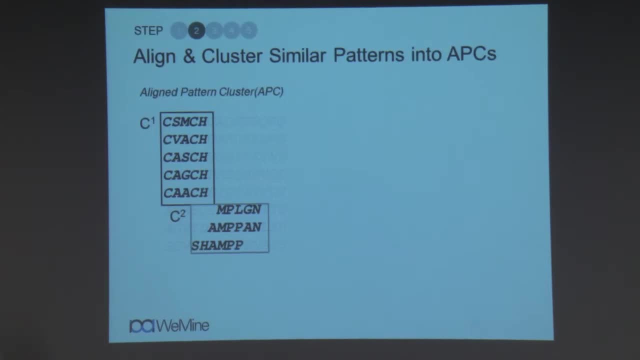 some kind of common functional framework so that we can see the commonality among these patterns. And then the APC contains co-related long random pattern implying similar underlying structure and function. And later we find out that yeah, it did relate back to the structure and function. 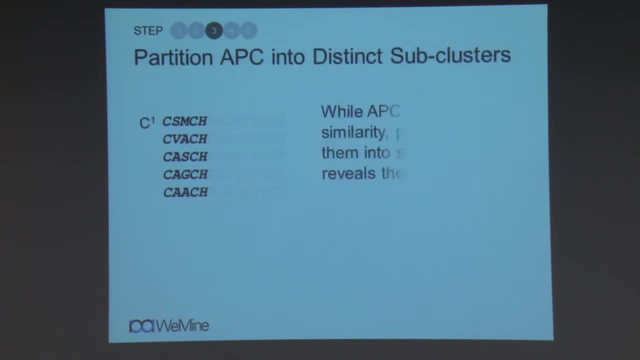 And then we can see the co-relativization of the molecules. Then we further partition them into and then using sub-information measure to show that they indeed can reflect the subtle class characteristic. For example, now we have an aligned pattern cluster. 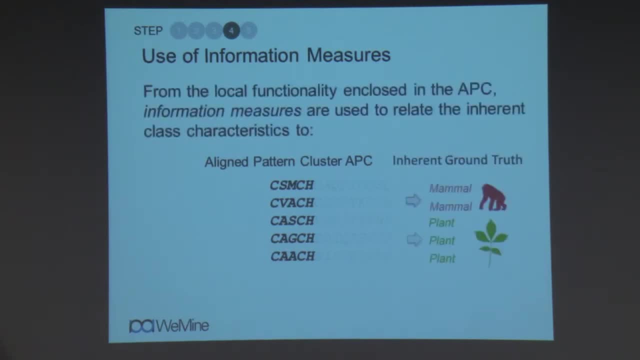 And if we bring back the ground truth, then we can find out which pattern right from the local functional group- now we look at the local functional- that within this local functional group we can find out what class, Then we find out that some pattern are connected to memo. 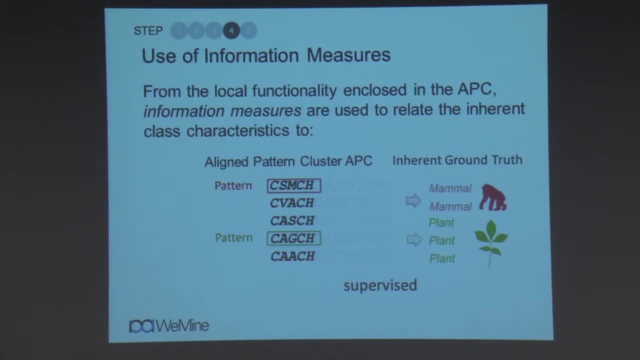 some pattern are to high plan. okay. So this is any sequence right, because the association of related back to the memo. If you look at the column in an unsupervised way, we don't know what is a class, but if we find a certain site, 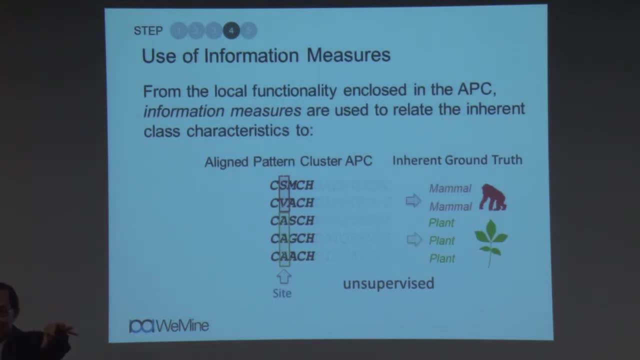 which is high interdependency with all the other sites. right, there's information measure can pick up those sites and you know that those sites contain MLO assets which are related to specific class. even class label are not there, Because what is a class? 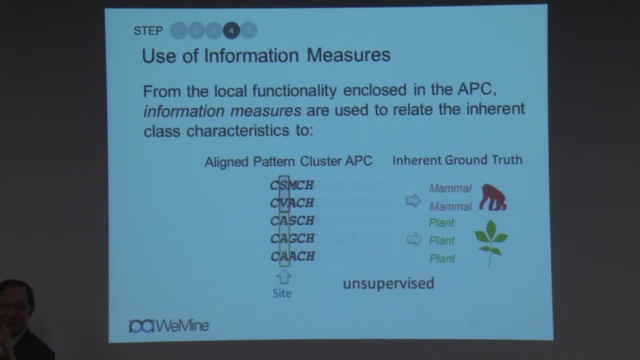 Class means that if we fix something, they're interdependent- right into certain group, okay, certain functional group. In a like manner, even MLO asset we can go to MLO asset. therefore, if you ask me for this important site, 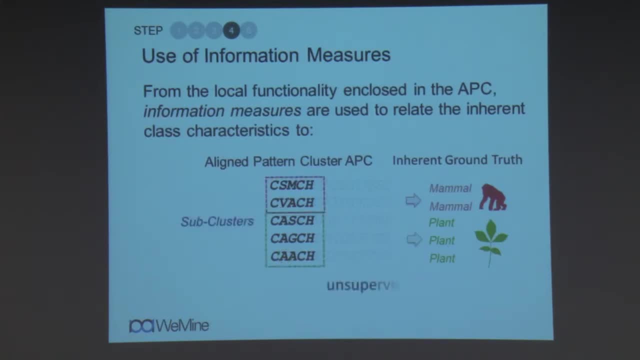 which MLO asset will be related to what class. Or, furthermore, we can find out which subgroup would belong to which class. This subgroup belong to memo and the other group belong to plan. So by co-occurrence, it means that if two patterns 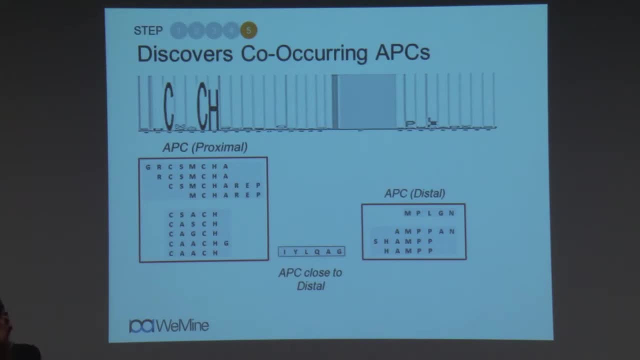 they always co-occur on a molecule. it indicate that they have some kind of joint functionality. It may cover their folding, their interaction or any way. So here we find out that these are co-occurrence APC, but these two are somehow co-occur. 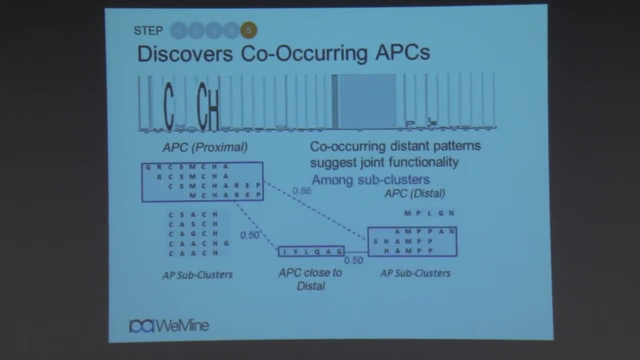 If you go at the sub-class level we also find out that these are co-occur. We can see that two co-occurrence group. it suggests that two group of molecule their co-occurrence functionality could be a little different at a distance. 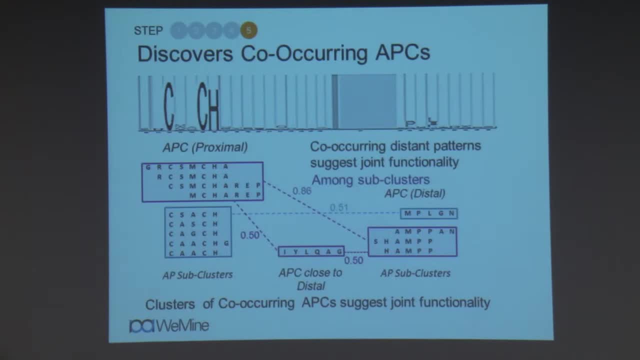 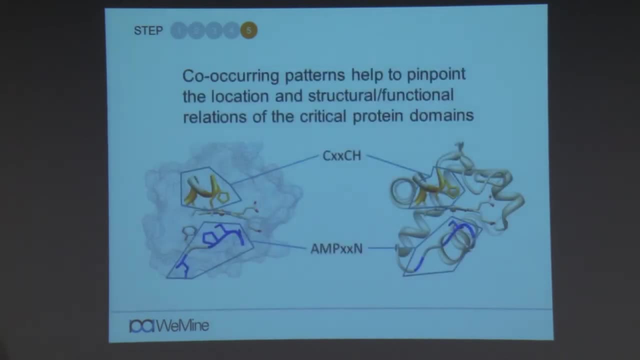 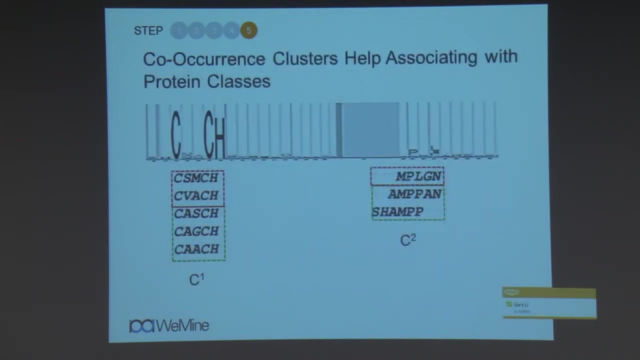 So the whole idea is we suggest some joint functionality When you're using the Raptor or other program. then you can see how those regions are related back to the structure and function- interacting energy, whatever of that- In a lay manner. 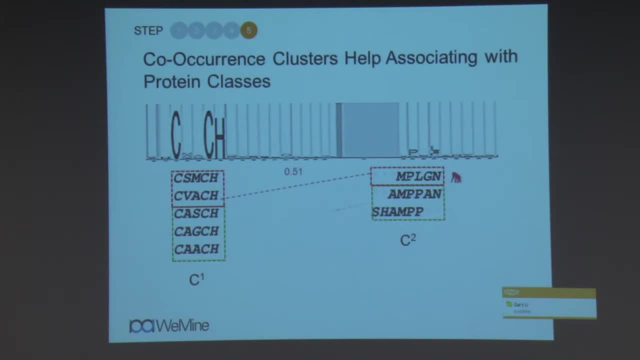 we also find out that some co-occurrence group related to mammal, other related to plant. So, in a nutshell, this is the methodology we have developed and we unified. We can, using co-occurrence measure to bring out those APC. 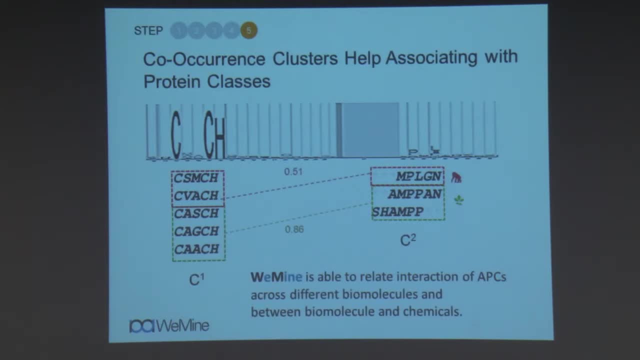 which is co-occurrence. We can also using another kind of score, like a chemical interaction score, to bring out those regions that can have interaction between protein and protein, protein RNA or protein and chemical and so forth. So now we give some case study. 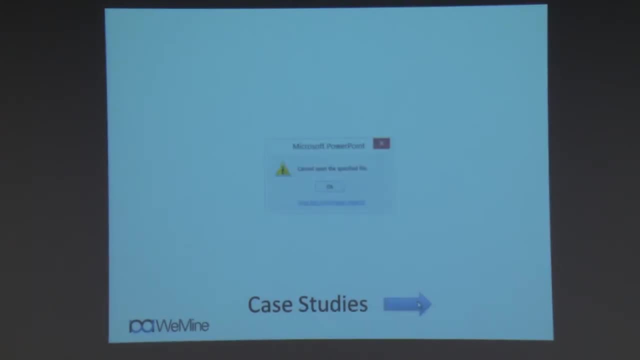 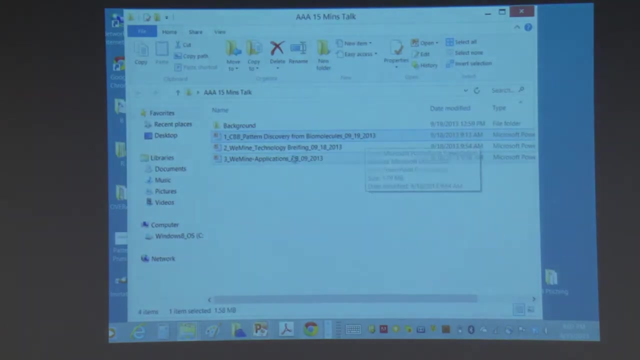 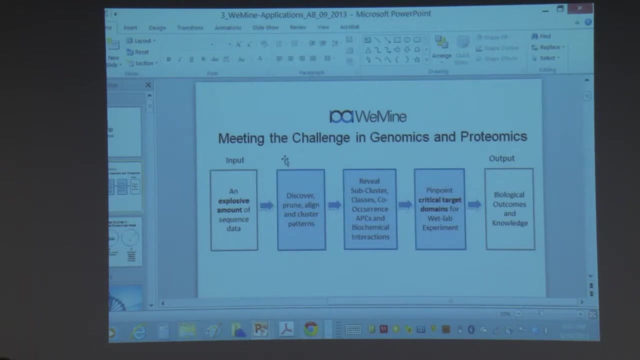 then I will end my talk. This is something Now application, Now in the classical, in the traditional method. so we have begin with a lot of data. Now in our method we discover prune and line and cluster pattern. 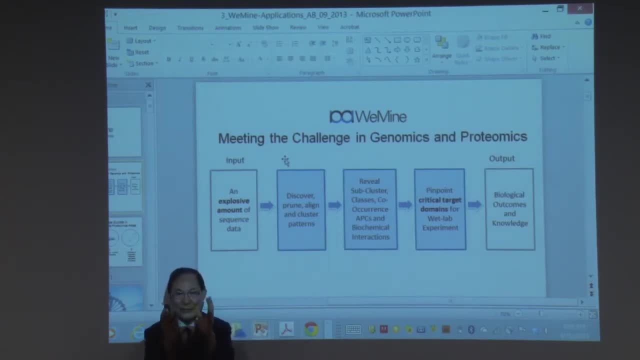 to bring the similarity functional unit together And then we reveal the sub-cluster, reveal the class co-occurrence and also biochemical interaction, And then we pinpoint the critical target domain for wet map experiment so that we can pass it on. 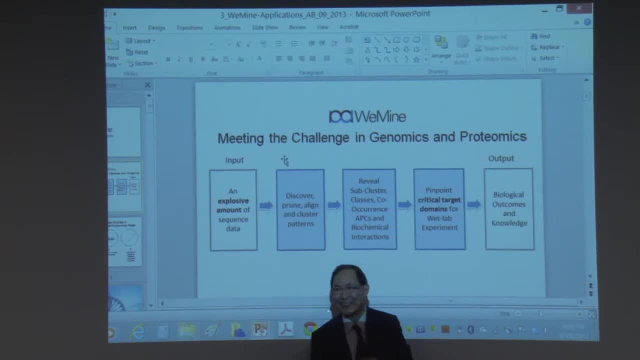 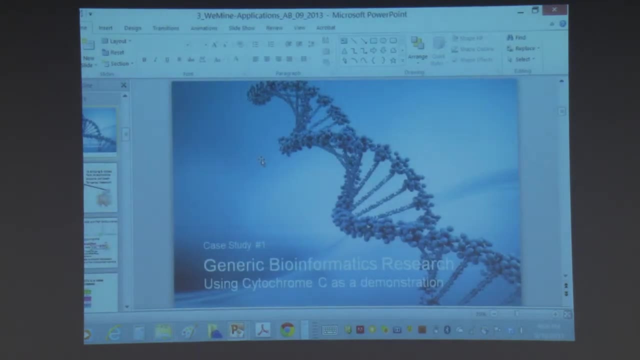 to the biology, to zero in, to confirm So this scientific method right Now, then in the. so now we begin with three. First, we would demonstrate using cytochrome C, demonstrate that this can be applied. 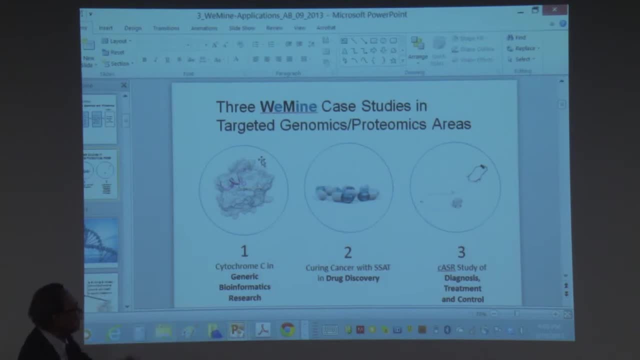 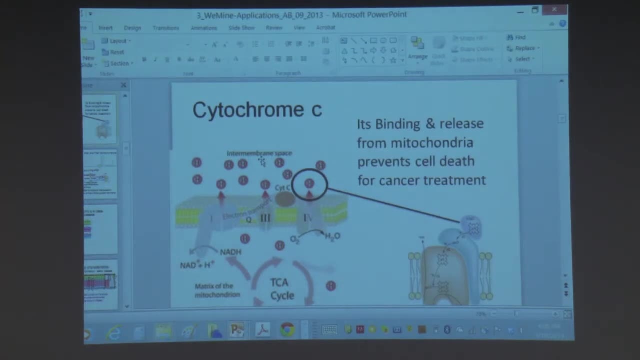 to genetic information research, Second, the drug discovery and thirdly in the disease treatment. Now I don't have to say any more about cytochrome C. It is very important. It's binding and released from the mitochondria. 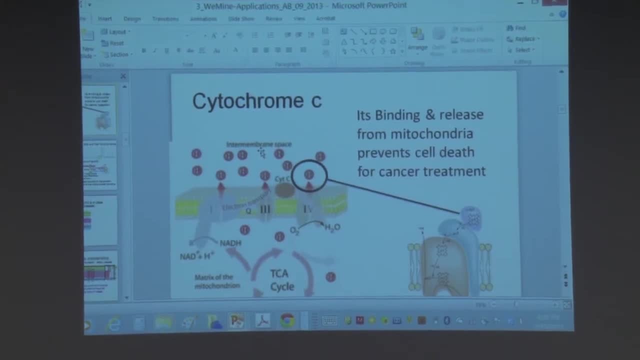 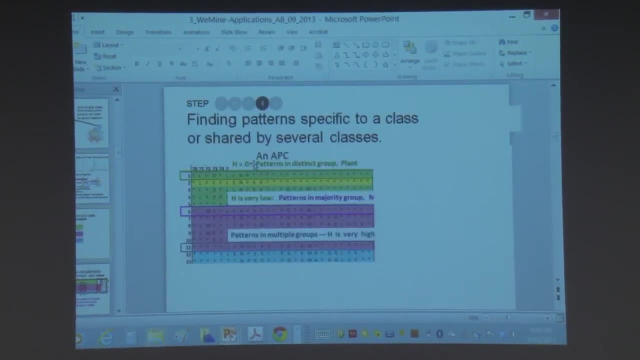 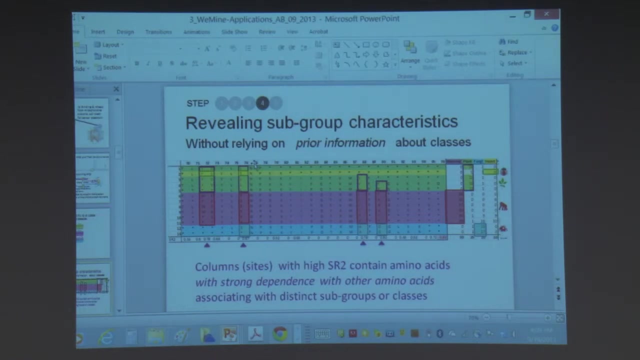 prevents cell death for cancer treatment. So this is the way we can find out how things co-occur. Now, here we demonstrate how can support. so I don't know what happened Now, so you lose the animation. 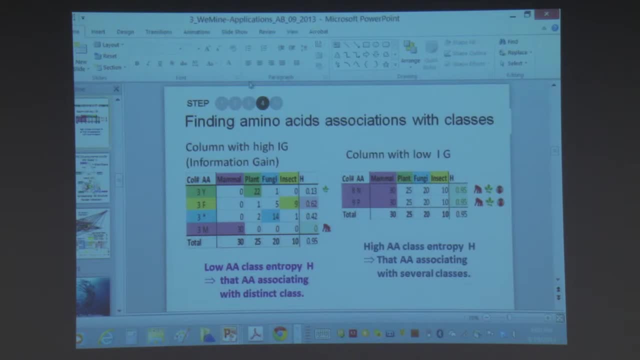 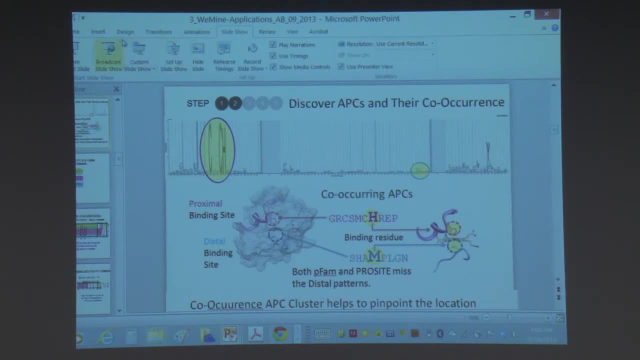 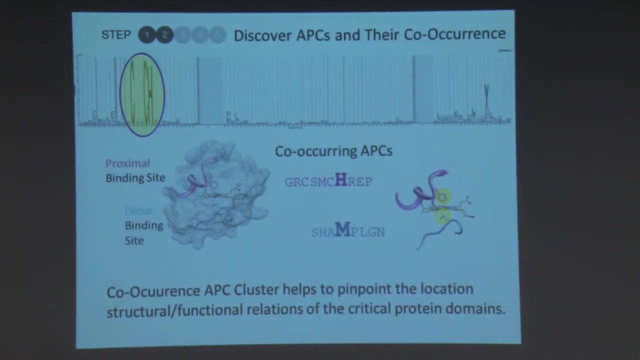 Oh sorry, Excuse me. Yeah, Sometimes you rely too much on high tech. High tech can betray you. Okay, Now here. first we found out that these are occur, and then we found out that they're embedded in there. 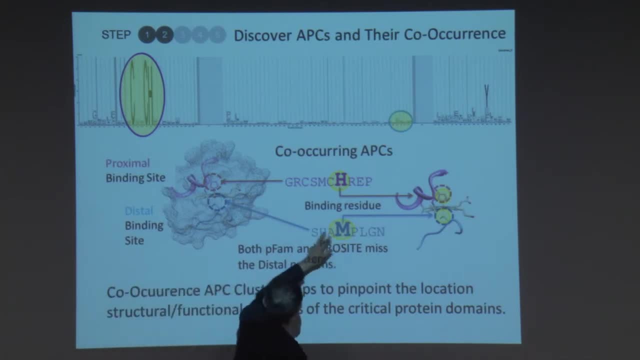 in your APC, some significant site which is very significant within this site, And both PFAM and POSI cannot find this because they only find M, but we found M right. They only find M because they only find the principal, because 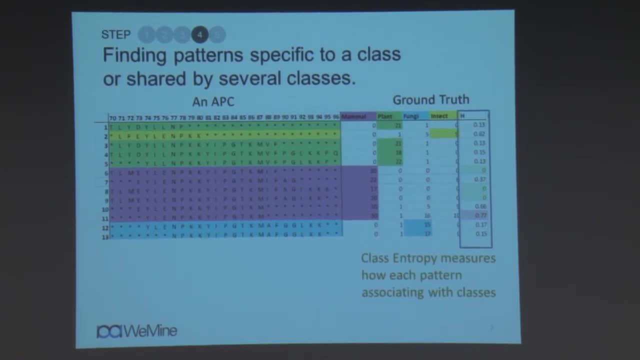 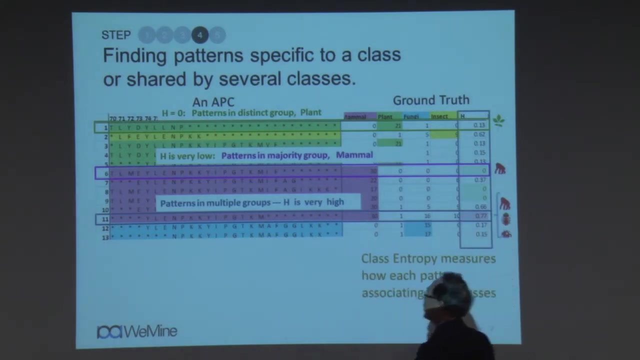 they're in this site. So, as you can see, these are some of the parameters that can be found and we can see how this is. These patterns are shared by three different groups, and one is specific for one group and the other group. 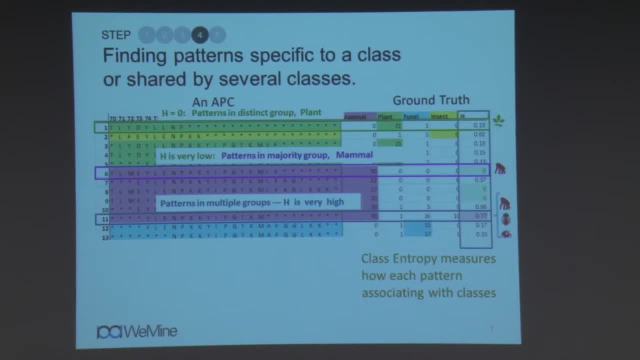 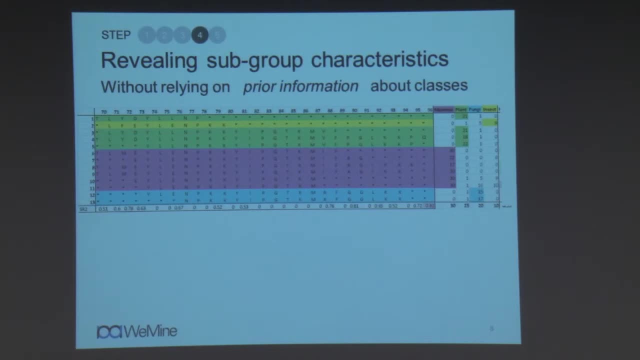 Automatically, then we can let the biology figure out why and then perform experiments to verify. Now, without any prior knowledge, with some kind of information measure, we are able to find a certain site that must contain some very distinct information, like this one: 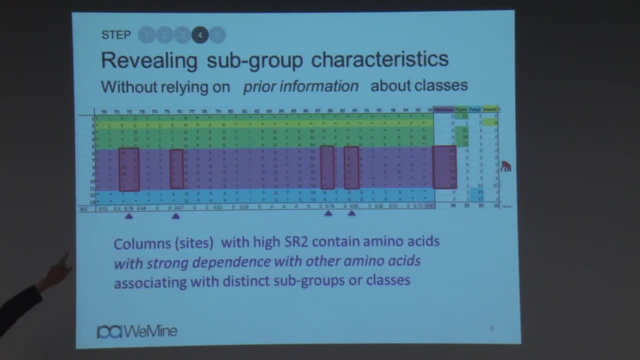 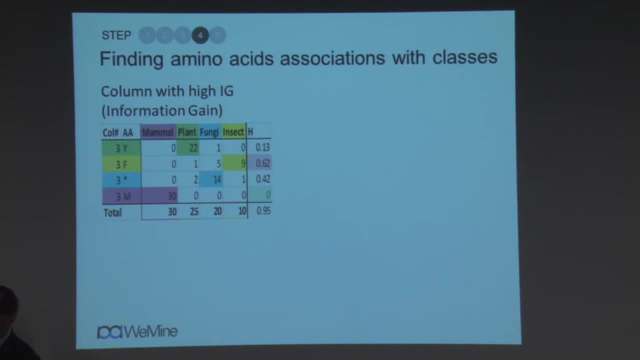 with very high interdependency measures. So for this group all E and A. they share with mammal, some with the insect, some with high plant and some with that. Automatically we are able to pick it up into some kind of class and review. 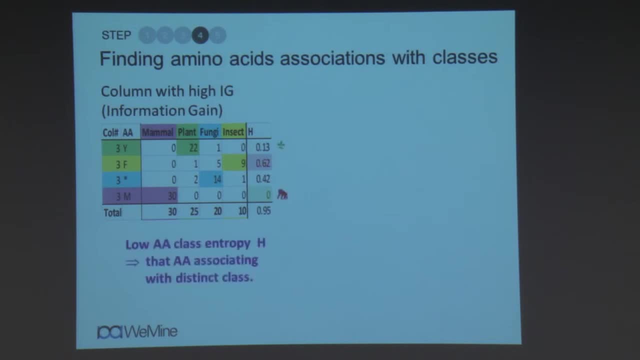 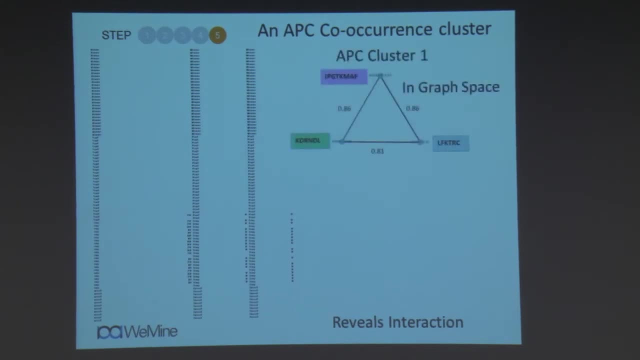 the underlying functionality of each class. Even we can go into the amylase acid level. I can skip this. Now, in a nutshell, we are able to find some kind of co-occur ABC. We can find it, map it into this graph space. 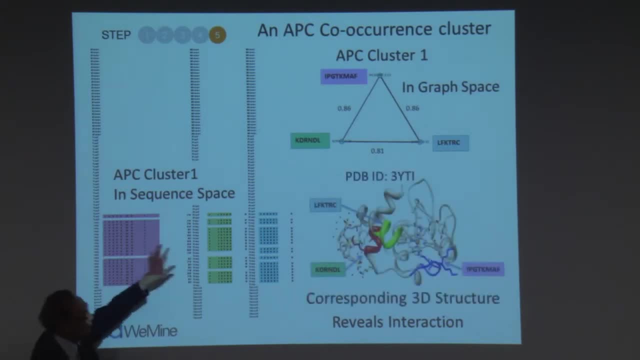 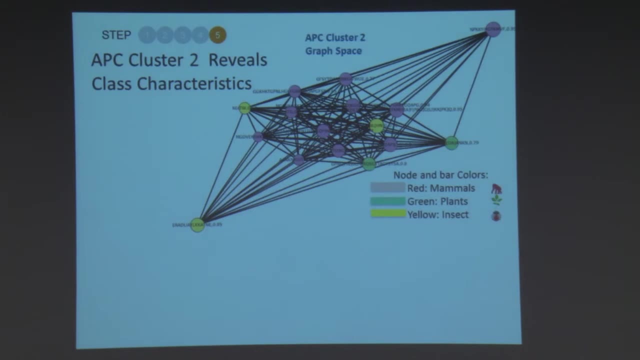 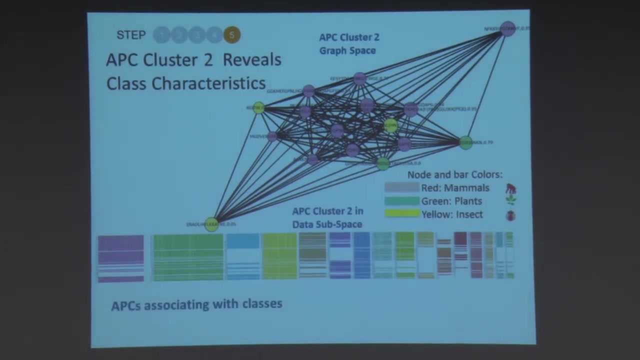 in a pattern space and also in the data space and back into the 3D space. So this is more very, very interesting. For example, once we find out this cluster, then we can find out that actually this group contains. 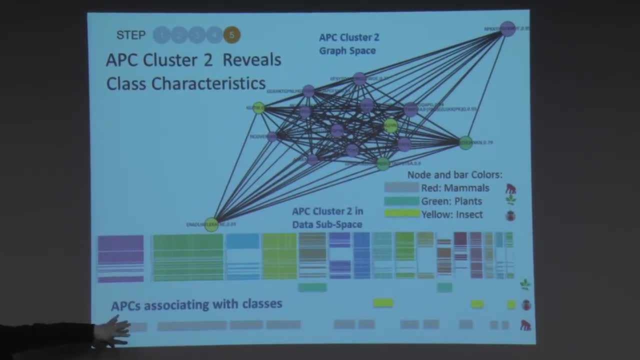 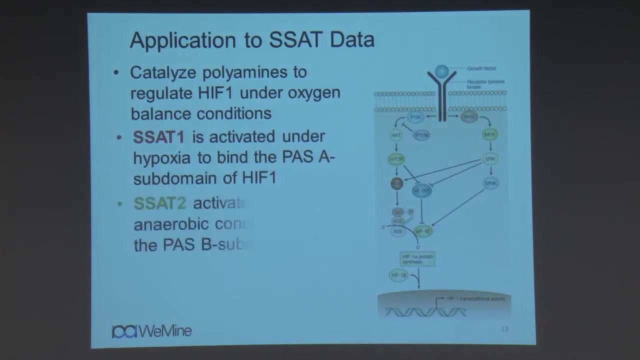 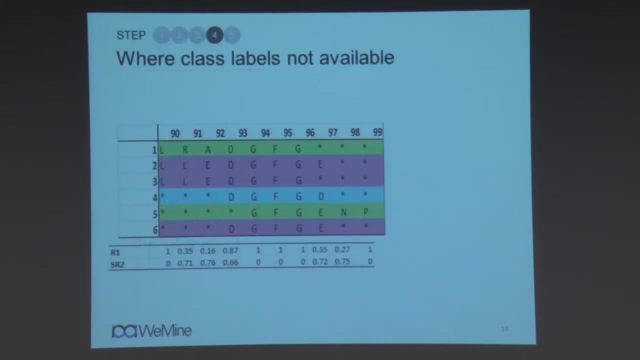 interlaced pattern. They span different domain. OK, So they may be a little different. And then we go into the drug discovery. Now this molecule related back to the killing of cancer. I do not want to go to the detail. 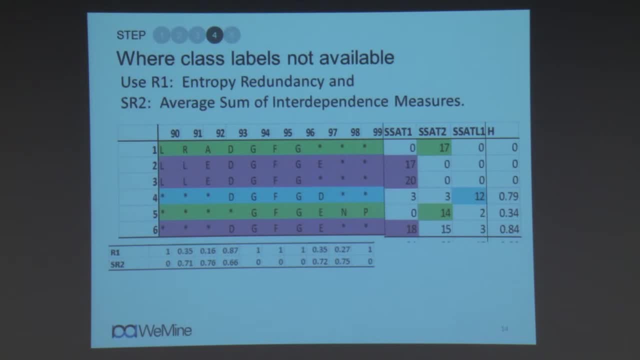 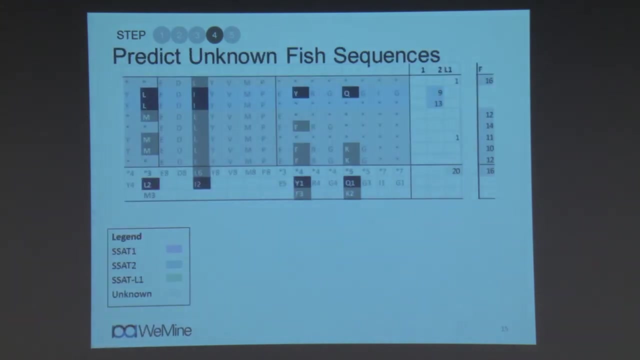 But by the same notion. we are able to discover some of the patterns And then we can associate back to this. You can see A, One class, E, another class and all that, And once we are able to isolate this functional group, 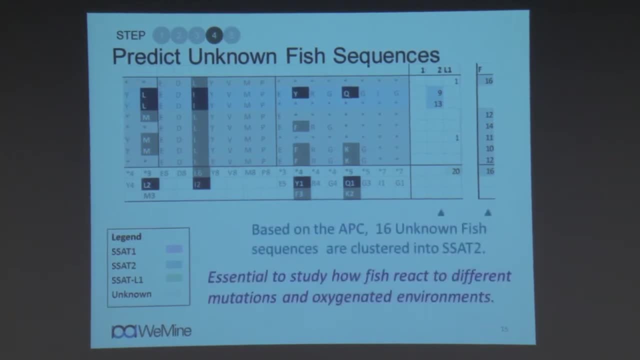 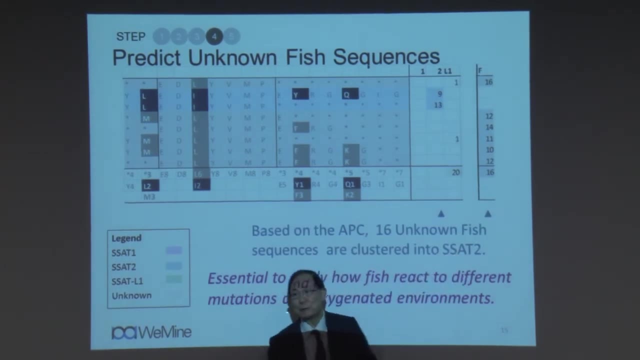 then there are some unknown features. OK, We can associate unknown features to which group, Like the 16 features are associated with set 2. And we call it semi-superwide. We use it unsupervised to find a group and then using that to pick up something related to that. 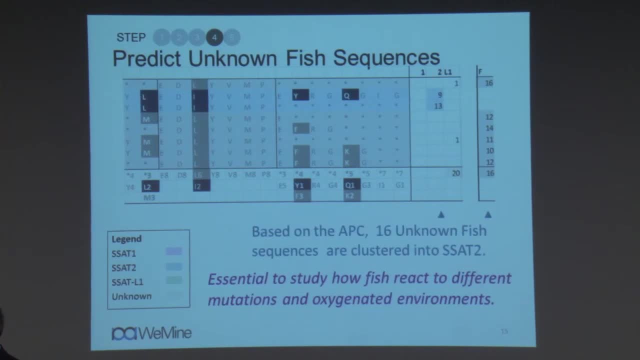 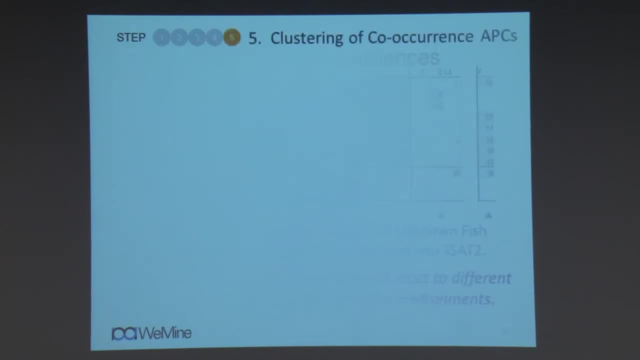 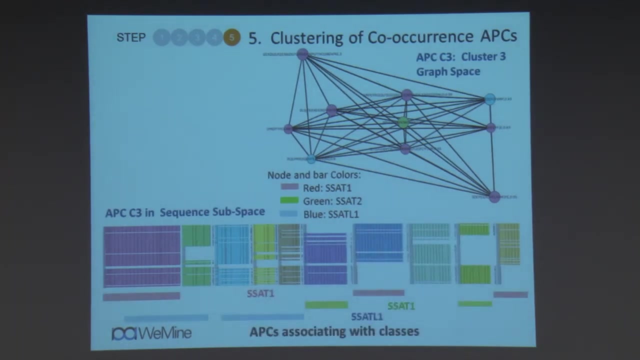 So if this is a cancerous data, right then once you, we don't know what does it mean, right? If you can find out certain group, then you can bring in other. So this is just further demonstrate You can find out the interlaced kind of co-occur pattern. 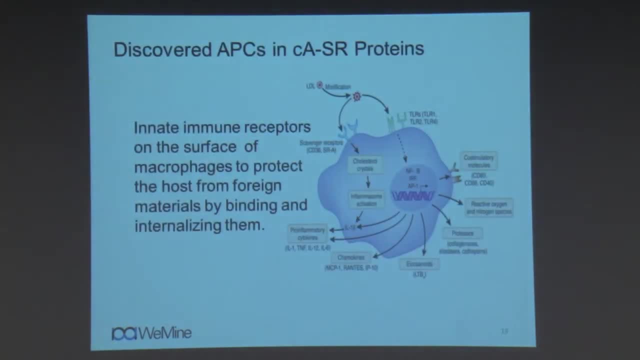 And relate back to the 3D. well Now, finally, we just show that we can also apply this to find out the region, the functional region, in a molecule from the APC rediscover. Now, these are two very interesting things. This is a very interesting molecule. 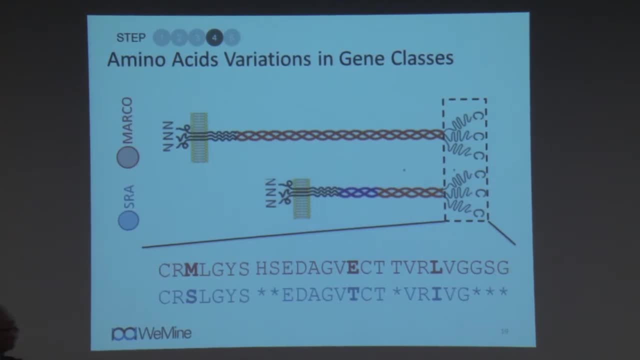 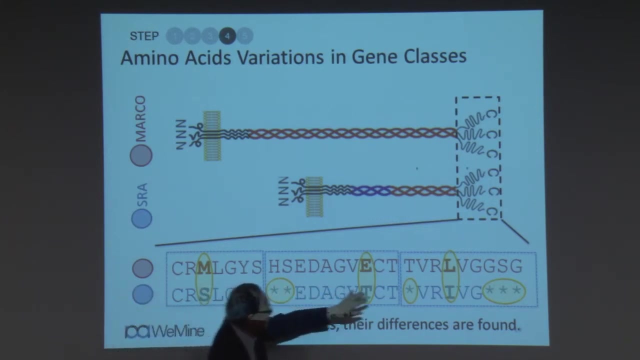 One is longer, the other is shorter, But the whole functional group is here. So again, there are two classes, But these are scattered along the long sequence. They are 500 bases long, But once we find out these three APC, you can see the differences very easily. 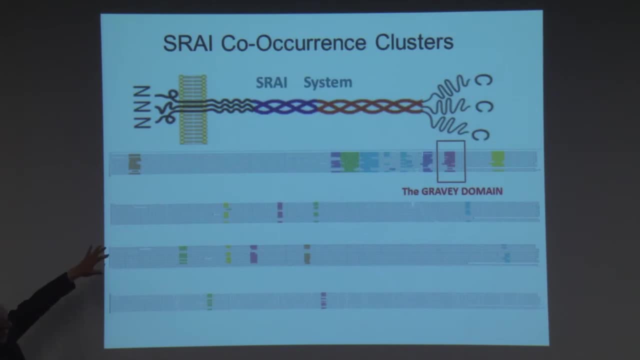 OK. Now if you want to plot the APC on the long sequence, you can see they span different domain. OK at a distance. Why? Because structurally, functionally, there are some intrinsic meaning there. So with that we certainly, I'm sure, the biologists. 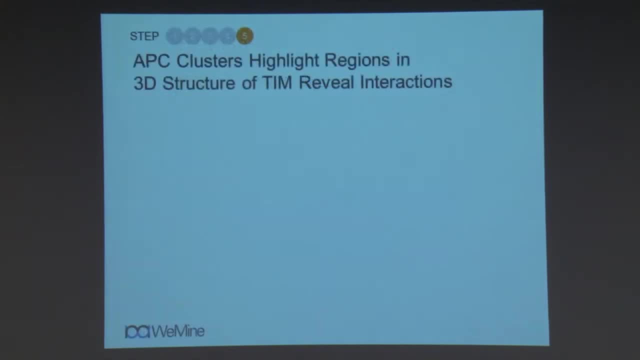 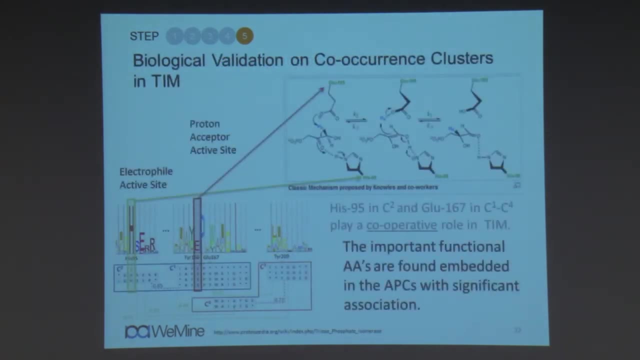 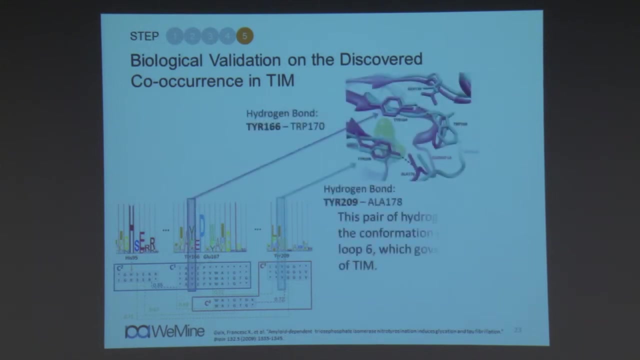 will be really happy to find out what, why. Now, just further demonstrate. From now on I just show you we are able to discover something worded, data by biologists and find from biological papers- And so far, OK, you can see, the key thing- are picked up. 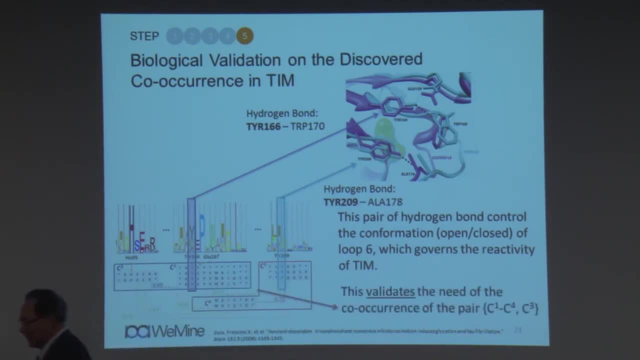 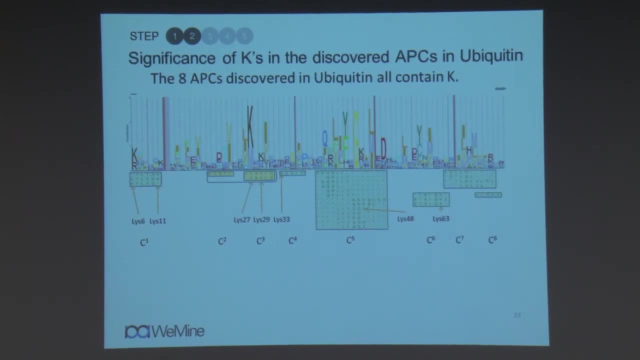 and then relayed back to the 3D. well, And so are these other group, And here it's very interesting: lysine Today we do lysine very much related to cancer, right, And only our method can discover all the lysines spanning. 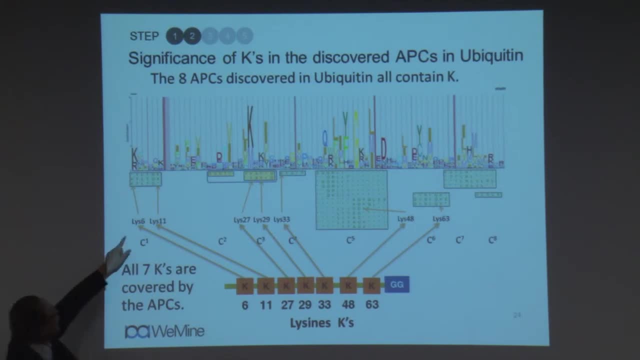 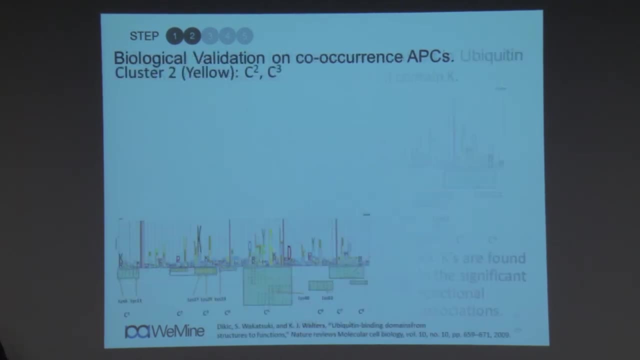 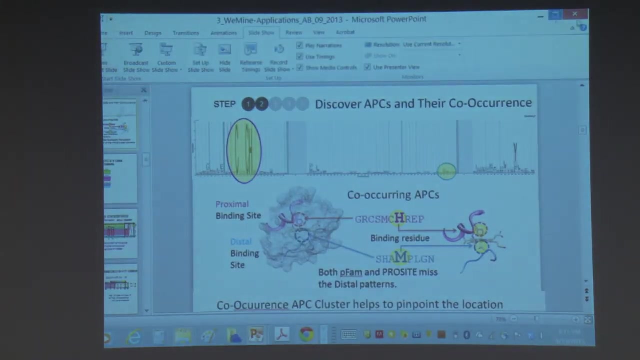 in this You can see that we pick them up, And two OK K are found in the significant functional association. And then, of course, there are many more Now. so I want to conclude Just for two minutes. I will conclude. 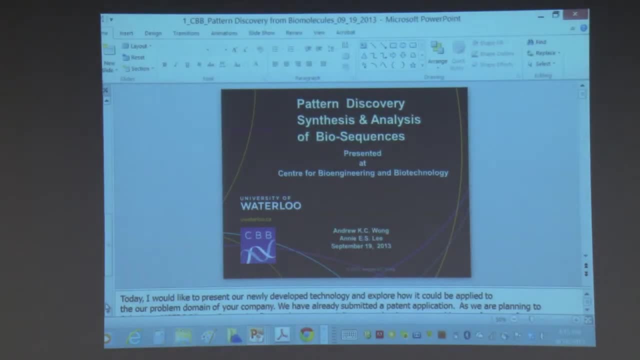 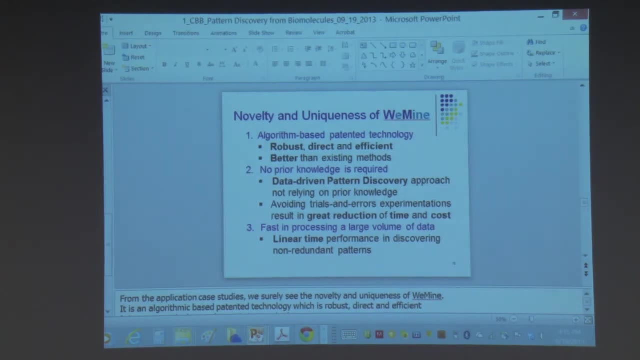 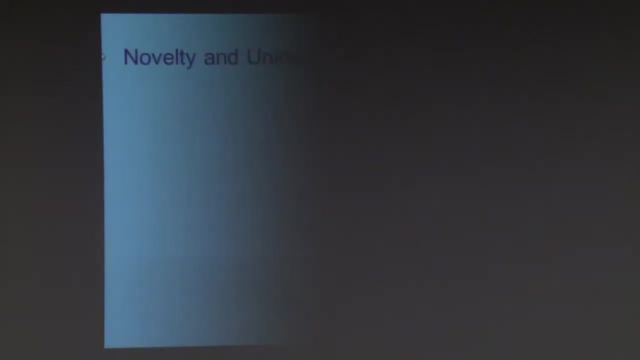 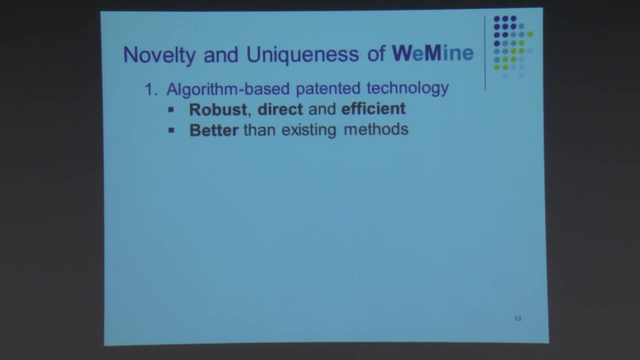 Let's see Now to conclude, And Now it's lawful and unique right, We are algorithmic-based, no, and robust, direct and efficient and based on statistic. So when we talk about pattern, with those one-hour- 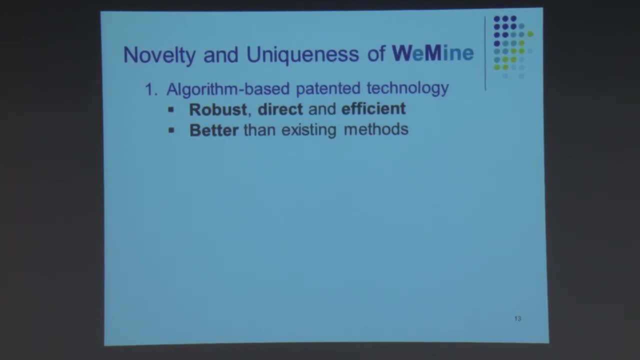 billion, billion chance. it cannot be random. Better than existing method fast. we have to do a lot of serious comparison in time complexity and in space complexity, And then they are different. driven not rely on prior knowledge. Avoid trying errors, experimentation. 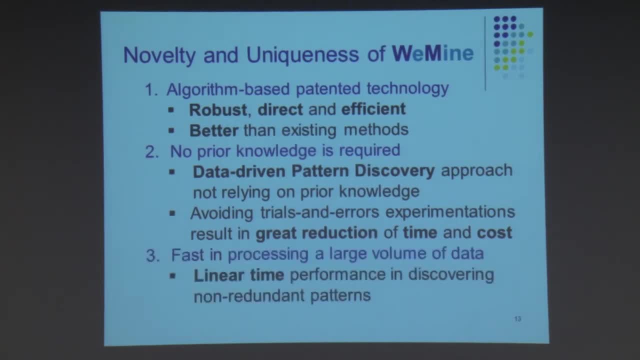 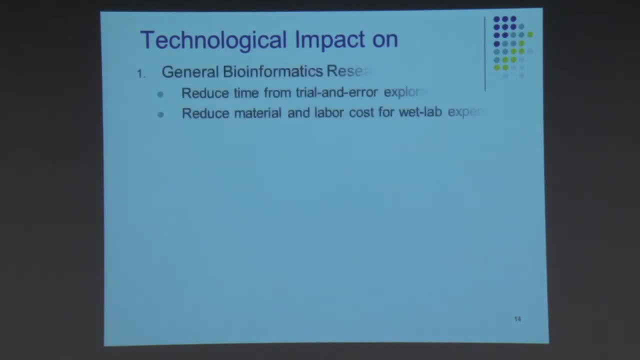 resulting in great reduction of time and cost. And fast in processing in large volume of data. linear time performance in discovering non-redundant patterns. So in bioinformatics we can reduce time from trial and error exploration, reduce material and labor costs for experiment. 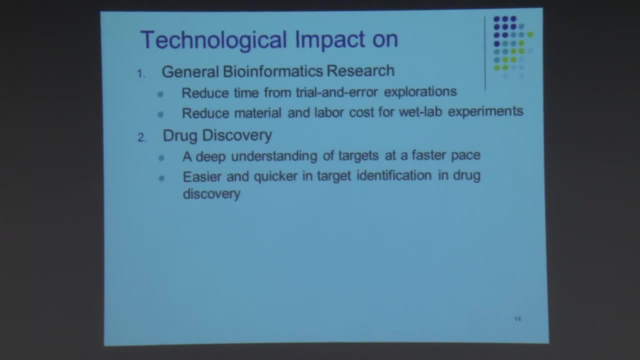 In drug discovery a deep understanding of target at a faster pace because we zero in from a lot of the ocean. you get to the island. then you can look at the island much more easily Easier and quicker in target identification and drug discovery. 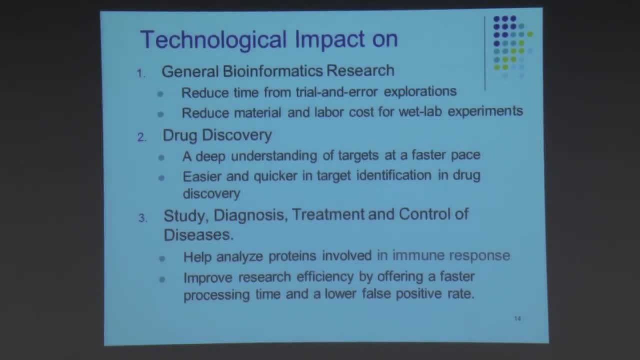 And study diagnosis and treatment that we can have a diagnosis of protein involved in immune response, improve research efficiency by ordering a faster processing time and lower force process rate. So, in summary, it is a unique process to allow biologists and medical researchers 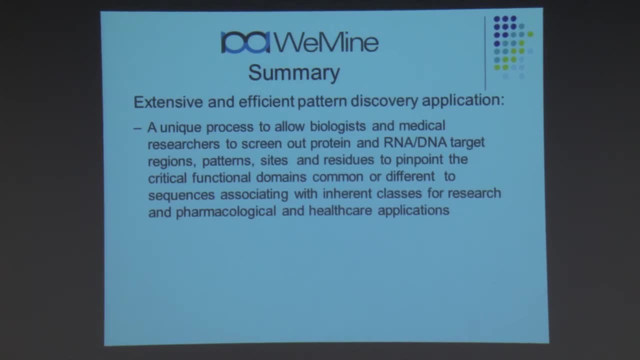 to screen out protein and RNA and DNA, target region, pattern, site and residue. to pinpoint the critical functional domain, common or different to sequences. So we can think of the study at the end of the year, the study and the trial. So this is the data that we can see and we can go back to. 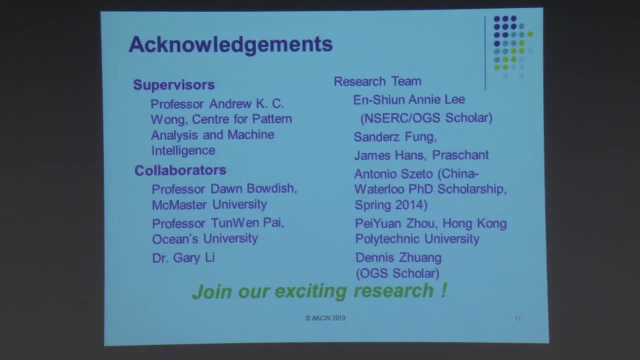 And this is the data that is being collected by the lab. Thank you all, Thank you. 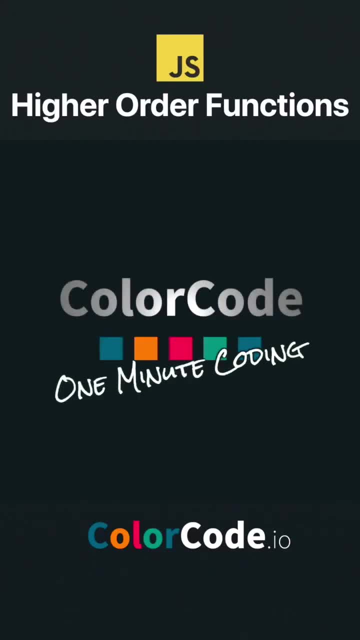 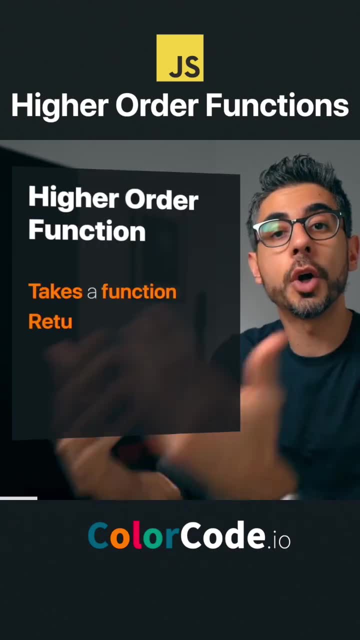 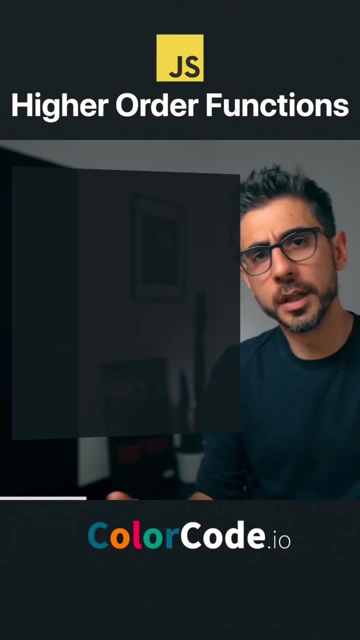 JavaScript: higher-order functions in one minute. A higher-order function in JavaScript is a function that either takes a function as a parameter or returns a function back to you. Any other function, a regular function, that doesn't do one of those two things is called a first-order function. Let's look at examples: SetTimeout. 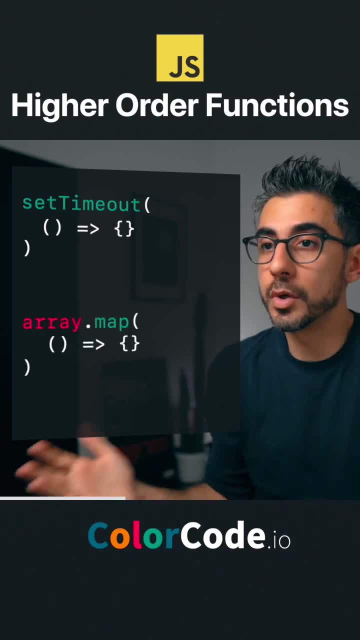 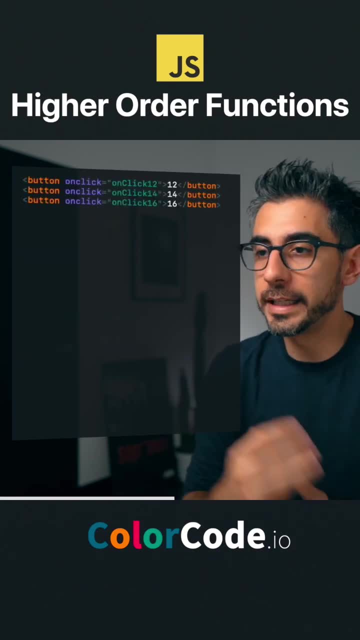 it takes a function as its first parameter. Arraymap also takes a function as a parameter. We do this in React all the time. How about one that returns a function? Say you have three buttons with three click handlers and all of them change the font size of the body depending on which. 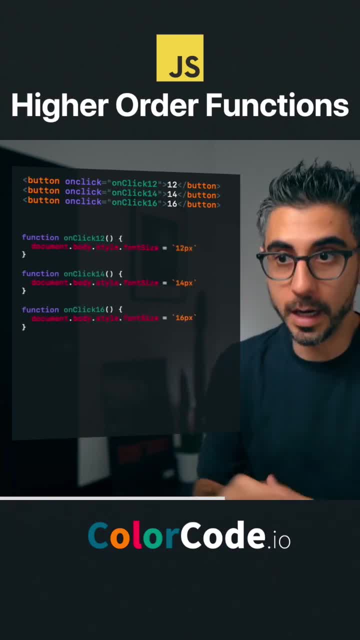 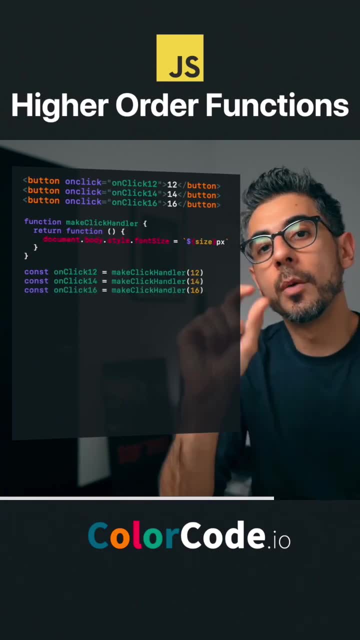 button was clicked. Instead of writing the function three times, you can write a higher-order function that generates those functions for you and returns them back to each button with their own specific size baked into the logic. This is something that we call a function factory, not to be confused. 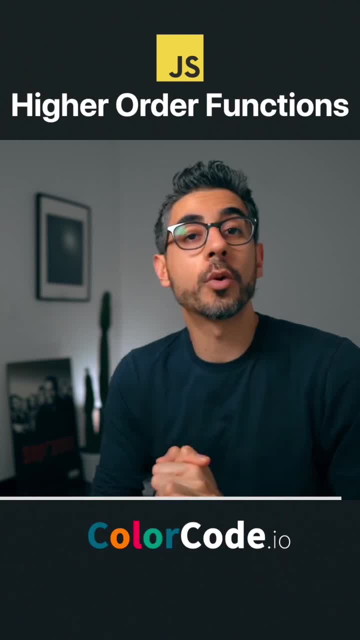 with a factory function. Better examples and how to use higher-order functions to your benefit over here on YouTube. But, by the way, have anything in your mind about how you can use Arraymap to generate many more functions in React? Let me show you an example. So if you have two player functions, I've got the first one and the second one and the last one and I can go in and see how I want them to work in React. I really like React, But I'm going to try and go in and see if there are any more functions. 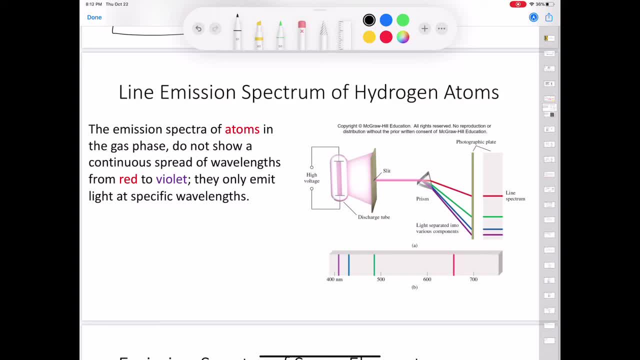 Einstein's work paved the way for the solution of yet another 19th century mystery in physics: the emission spectra of atoms. Ever since the 17th century, when Newton showed that sunlight is composed of various color components that can be recombined to produce white light,